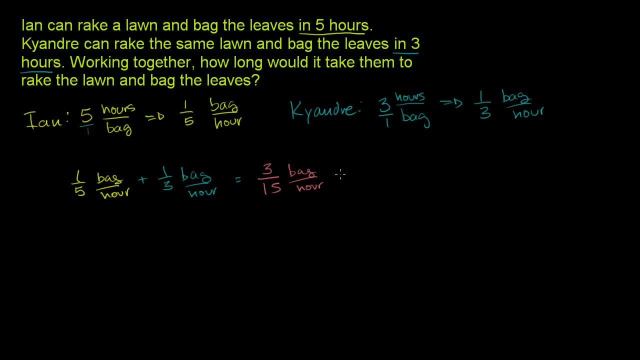 want to keep the units here: bag per hour. And then 1. third is the same thing as 5 over 15 bags per hour. So when you add them you get 3 plus 5 is 8.. So this is equal to 8 over 15 bags per hour. 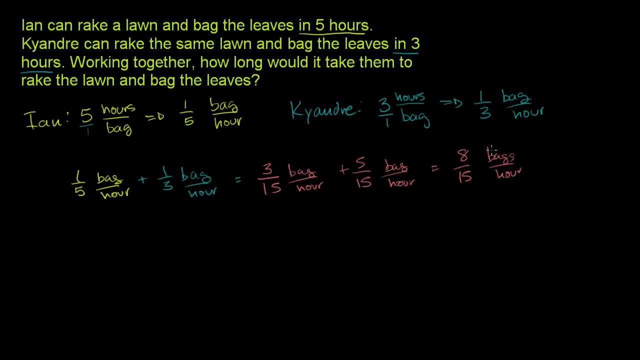 When I say bag, I mean all the stuff: rake, lawn and bag The whole tasks per hour: 8, 15ths of a task per hour. So, working together, how long would it take them to rake the lawn and bag the leaves? 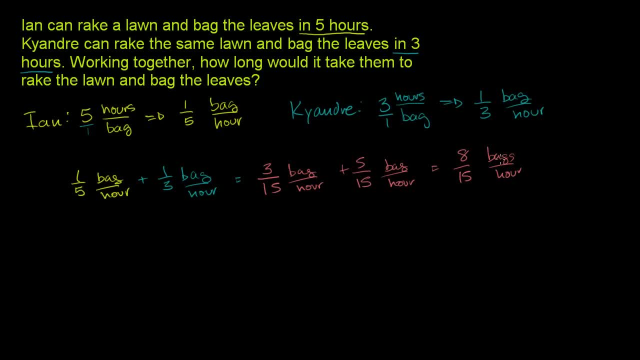 Well, this is how many of the bagging they can do per hour. You can invert this. So if you invert that, you get this is equal to 15 over 8 hours per bag. Or if we want to write this as a mixed number, this is equal. 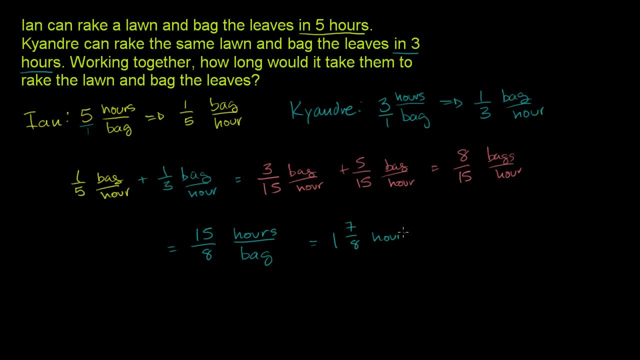 to 1 and 7 eighths hours per bag. Let me write it like this: 1 and 7 eighths hours, And if we really want to get a sense of what 7 eighths is in terms of hours, we can multiply it by minutes. 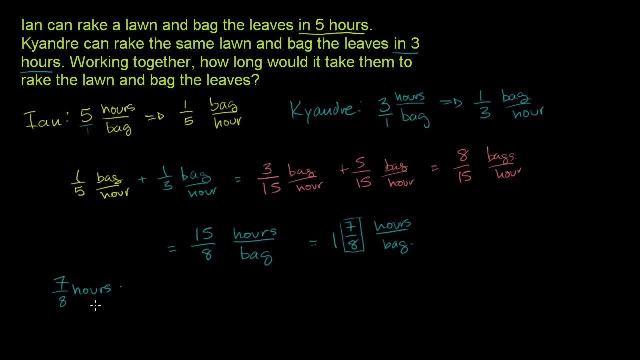 So 7 eighths hours times 60 minutes per hour, And let's see what we can do here. 60 and 8 are both divisible by 4.. 8 divided by 4 is 2.. 60 divided by 4 is 15.. 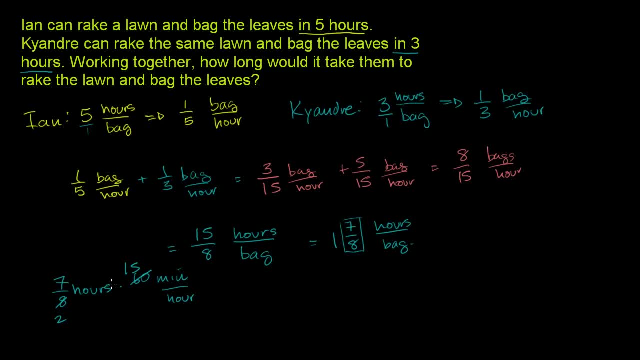 7 times 15 is. Let's see, 7 times 15 is 7 times 15 is. 7 times 10 is 70 plus 35 is 105. So this is equal to 105 over 2 minutes, which is equal to. 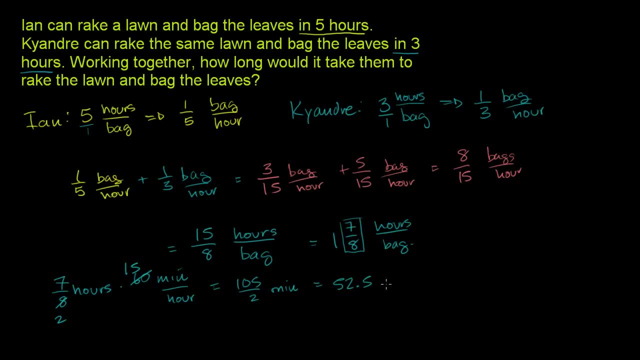 what 52.5 minutes. So as a combined effort, it will take them 1 hour and 52.5 minutes to do it together And we're done.